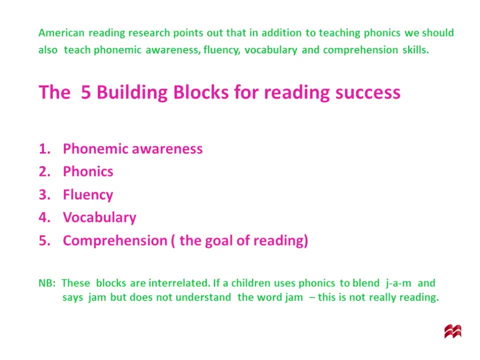 The fourth is vocabulary. We have to ensure children have a very strong vocabulary And five understanding- Understanding, as comprehension is the goal of reading. So these blocks are interrelated. For example, if a children looks at the letters j, a, m and says jam, using their phonics knowledge. 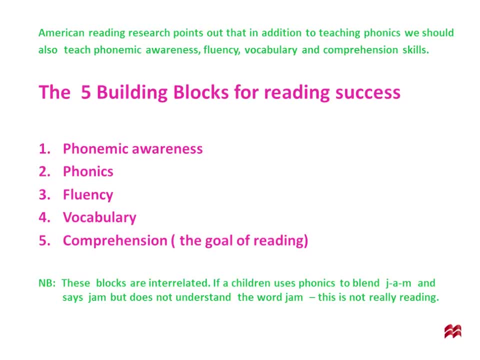 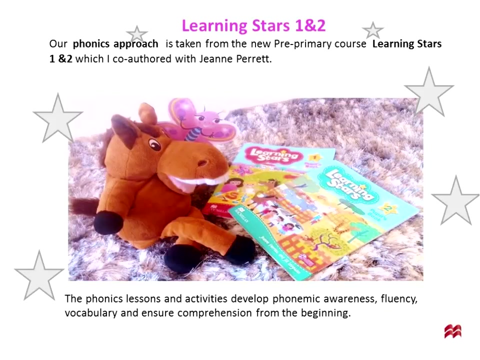 but does not understand the word. they're lacking vocabulary. this means if they're not understanding, this is not really reading. OK, So our phonics approach is taken from the new pre-primary course, a high-level course, Learning Stars 1 and 2, which I wrote along with Jan Perret. 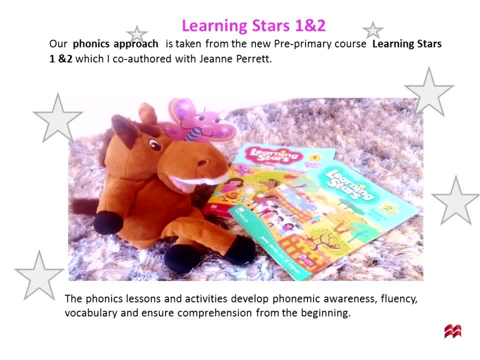 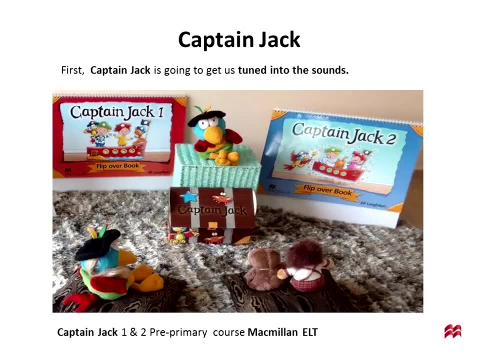 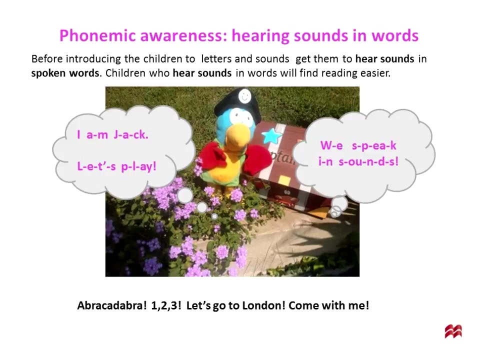 And we have integrated the five skills, So let's get going. OK, Captain Jack is also going to help us Now. he's going to start and get us tuned into the course. The sounds: Are you ready, Jack? OK, Before introducing the children to letters, we can introduce them to hearing sounds and words. 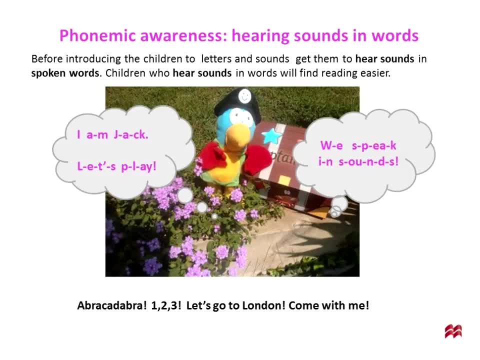 We're speaking sounds. I am Jack. Let's play. Children who hear sounds and words will feel will be much easier. So let's go, Jack. let's go. Abracadabra One, two, three. Let's go to London. 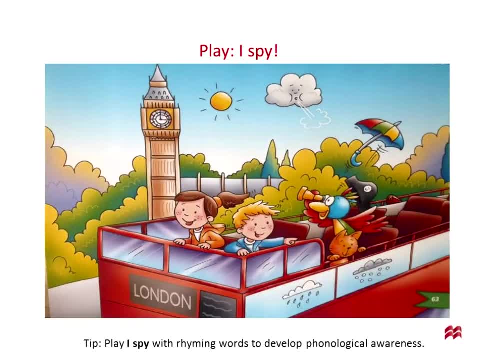 Come with me. Oh Look, Jack is in London And he's playing his favourite game with his telescope: iSpy. iSpy is a fantastic way to develop phonological awareness. OK, iSpy, a word beginning with B, Big Ben. 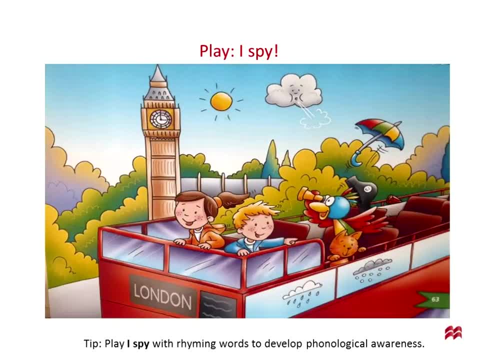 Bus iSpy, a word ending in M London Sun iSpy, a word with the middle sound A Ah, Sun Bus iSpy, a word that rhymes with cat Jill, Cat. Yes, Two seconds. We've had a few. 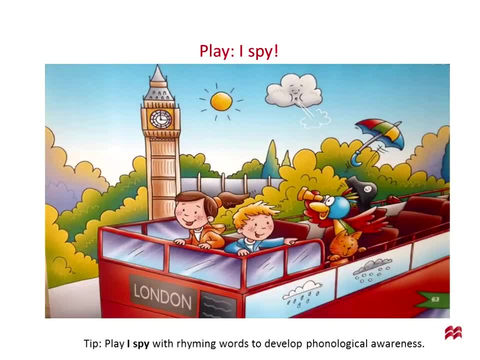 Hello, Sorry to interrupt. Sorry, We've had a few people just saying that you're coming through a bit quietly. Could you try, Right, just turning your volume up on the microphone and just maybe moving the microphone a bit Nearer your mouth. 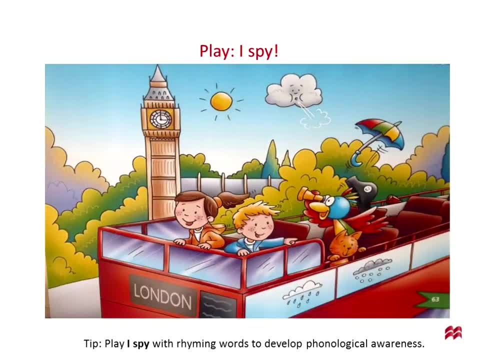 Or adjusting it slightly, Sorry to OK, Is this better? Let's just ask: Is this, Is this better? Can you hear me? Can you tell me everyone if that's better for you? Just say a few more words, Jill, and then we'll find out. 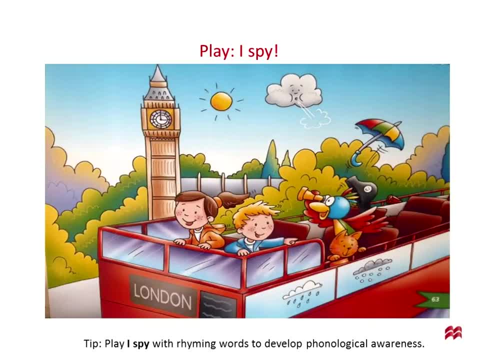 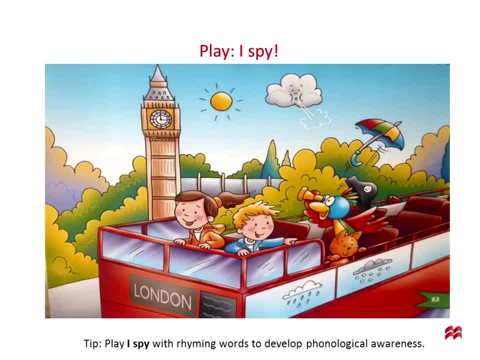 OK, OK, OK, OK, OK, OK, OK. Oh, Jill, you have to press the talk button as well. now, I wasn't hearing you. then If you press talk underneath your video, Right, Yeah, you're back. 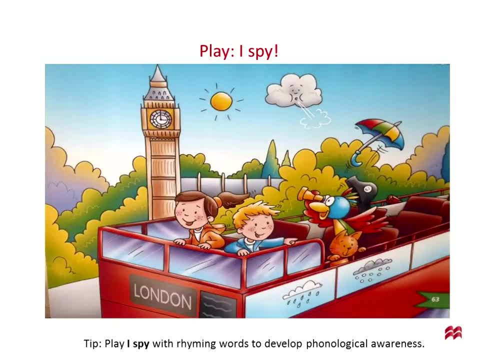 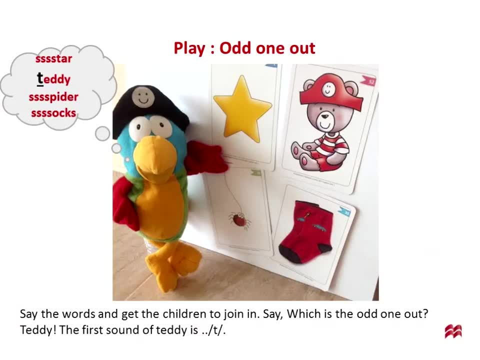 OK, Cool, We're back here. All right, I'll go again, OK, Good, Right, OK. Now Jack has another game for us. This game is Odd One Out Now we encourage the children to listen to the first sound and point to the flashcards. 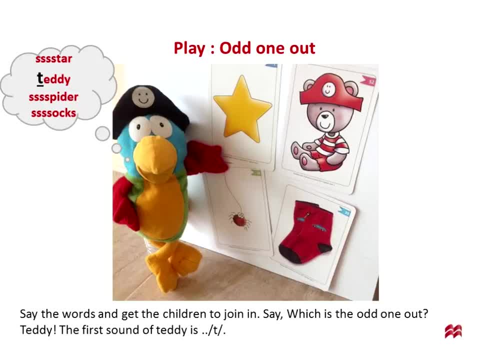 Star Teddy, Spider Socks, Which is the odd one out, Which is different: T Teddy. Teddy begins with T Fantastic. We have one more activity to develop Hearing sounds in words when you make awareness. OK, We can teach the children pre-reading skill. 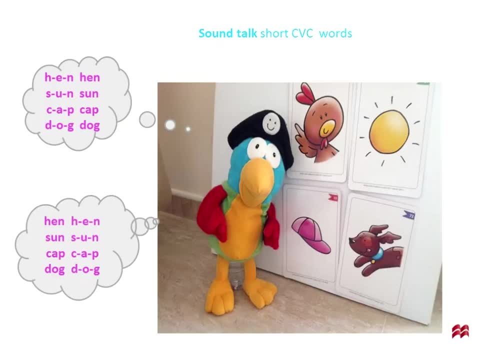 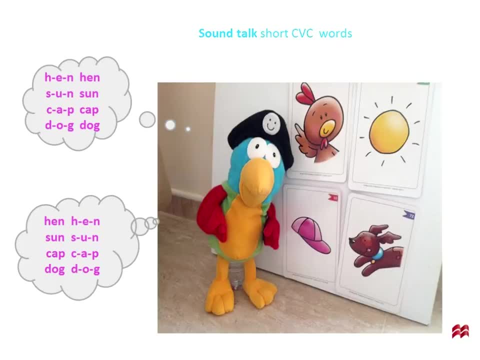 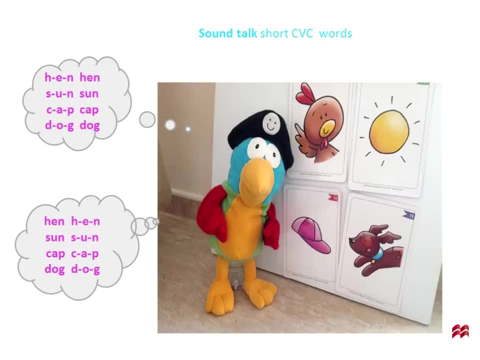 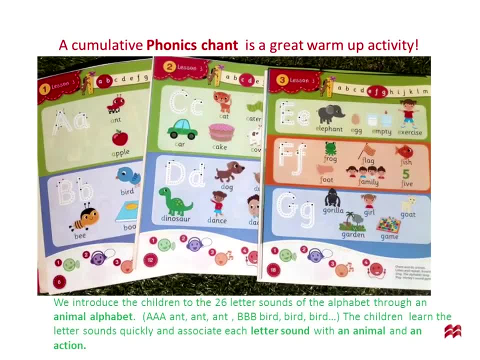 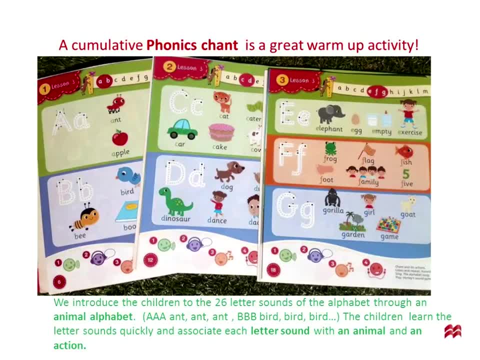 And the children learn an animal alphabet. Okay, this is a cumulative phonics chant that you could do in your class. There are two phonics lessons in each unit, So this is the first phonics lesson and you can see on the banner at the top. we begin with a, b and in the second unit, k, d. 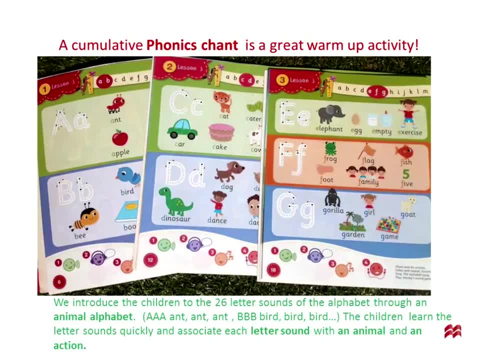 But this is cumulative, so we're always adding on. So let's try our phonics chant with animals. Are you ready to join in and do an action? Okay for unit one: Ant, ant, ant, b b b, bird, bird, bird. 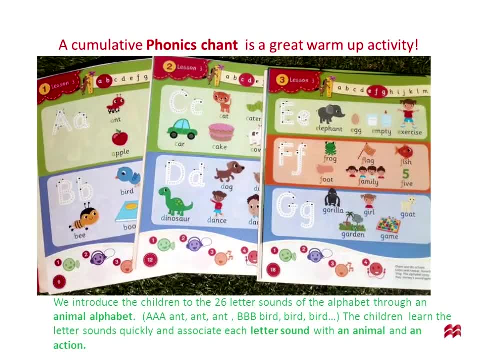 And then in unit two, before we add k and d, we revise A, a, a, ant, ant, ant, do the action. b, b, b, bird, bird, bird, k, k, k, cat, cat, cat, d, d, d. 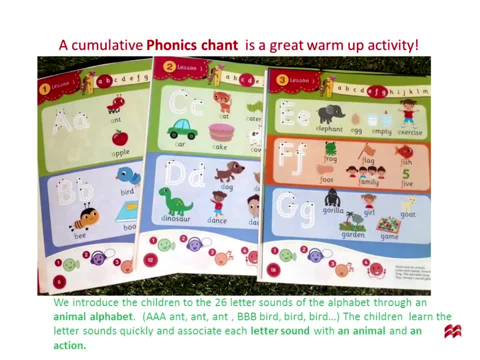 Dog, Dog, dog And so on. This is how we learn the letter sounds cumulatively In unit three. before we're going on to a, f, k, the children revise a, b, k, d, And it's a lovely warm-up activity. 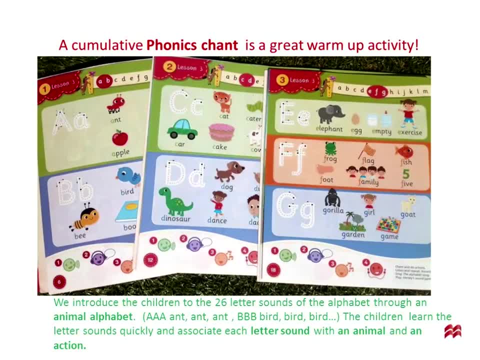 Now in this first lesson you can see, we build a strong vocabulary and we practice later formation and we also teach the children the letter name. The children are taught the concept that each letter has a name and a sound. They do this, they pick this up quite quickly and they do the letter names through the alphabet song. 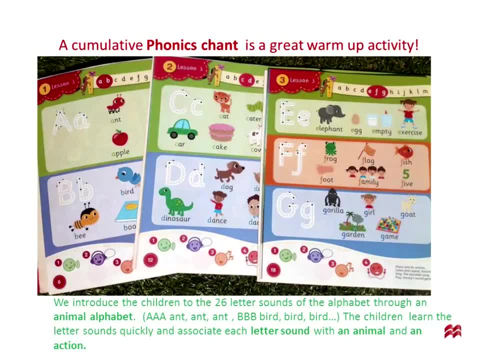 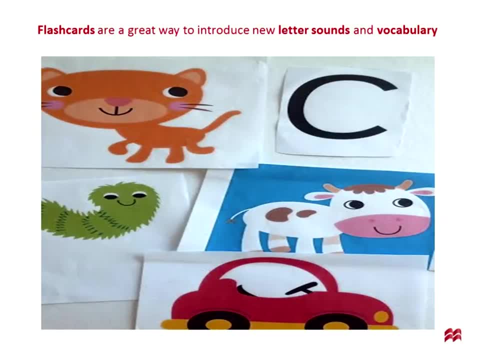 Okay, Now we're going to look at how we can teach the initial sound k K. Flashcards are a great way to introduce new letter sounds and vocabulary. Now we can show the children cat and get the children to say cat. 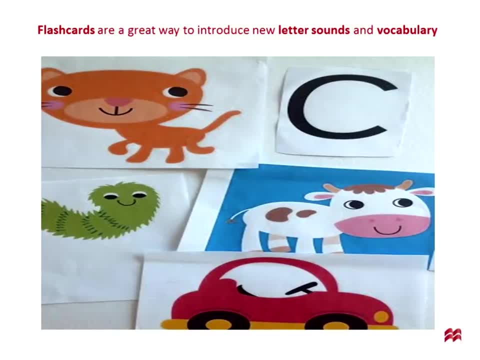 Cat begins with k. Now we can flash the flashcards in sequences and get the children to say cat. We can teach the children to say cat when they see the picture and k when they see the letter. For example: cat, cat, cat. 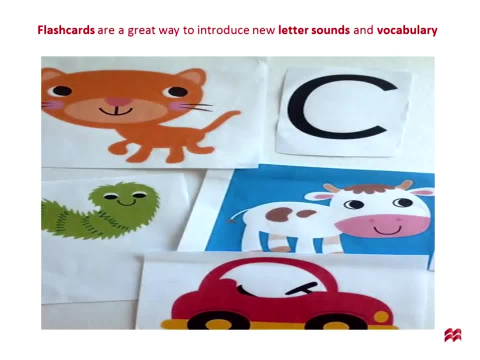 K k k Cat cat cat. K k k K cat k Cat. k k k Cat, cat cat. And we can do this for more words that begin with k. 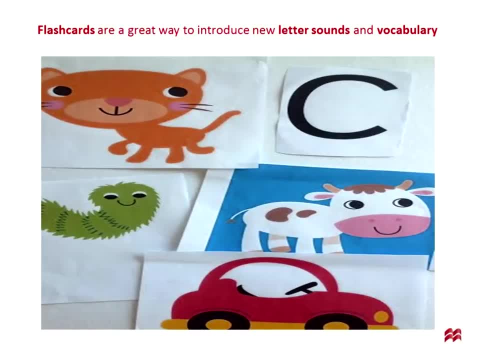 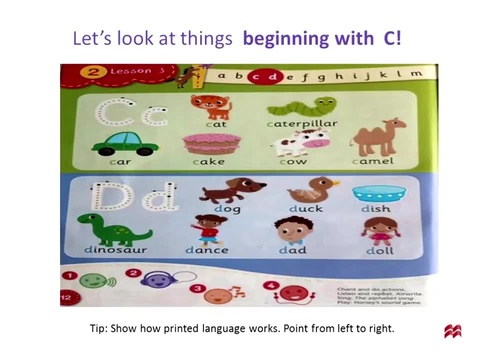 For example, Caterpillar cow car. Now we can put the flashcards on the board and write the word under the flashcard, Maybe putting the first sound in a different colour. okay, Now we want to show the children how printed language works. 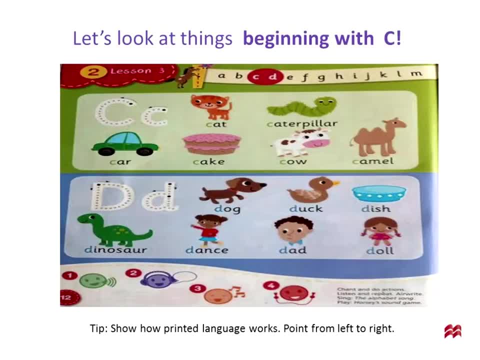 And it's very important to point to the words from left to right. Okay, so we get the children to listen first and we model pointing and then we get them to join in. First I would say: okay, how many things can you see that? 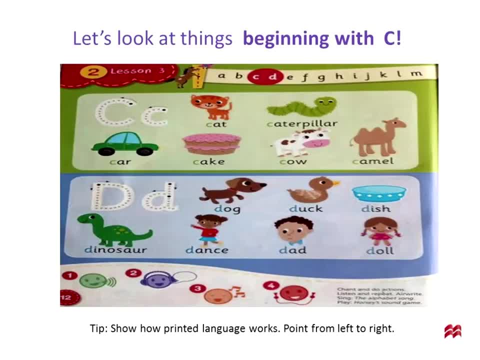 begin with k One, two, three, four, five, six. Good, How many words can you see that begin with k Six. What colour is k? Green. So you're really getting them to focus on the word Cat, caterpillar, car, cake, cow and camel And you would get them to repeat: 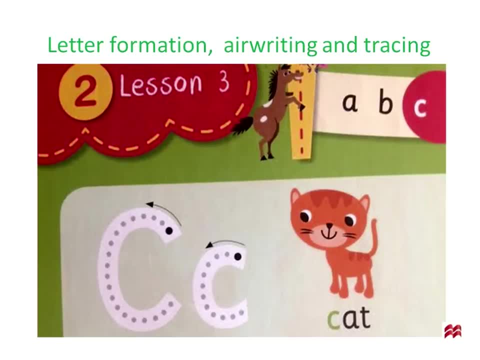 Now then horsey. No, no, horsey's not yet, Sorry. Now what we can do is we get them to air-write the letter, So we teach them capital K and small k. So we would write capital K on the board with the starting dot and the arrows, and small k with 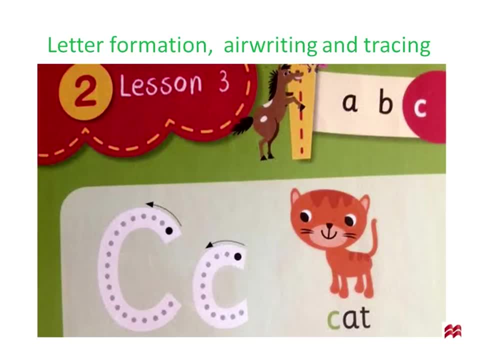 the starting dot and the arrows and show the children how to write the letter k, And then we would get the children to write the letter k in the air. Okay, you ready, Fingers in the air. So let's do that. 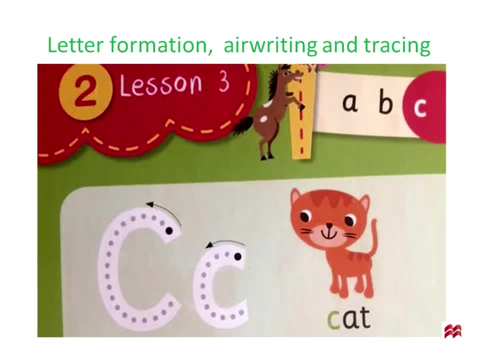 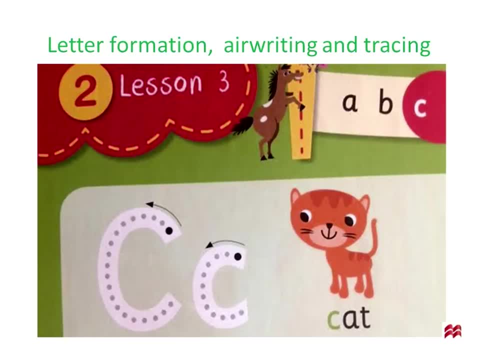 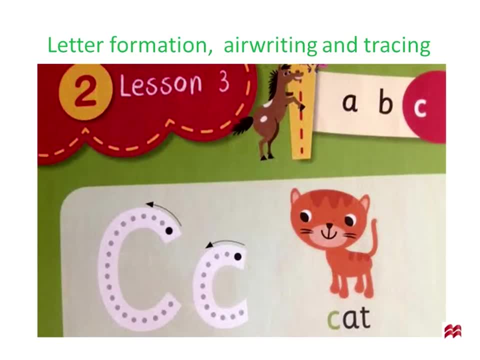 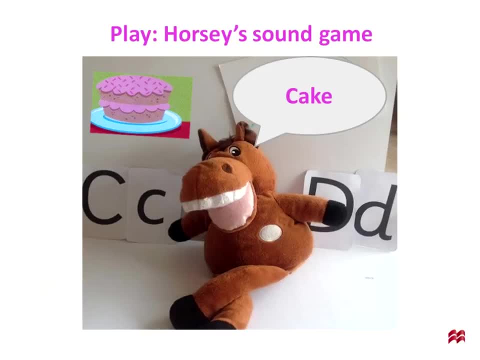 is the way we write capital K. Ah. now Horsey. Horsey wants to play one of his favourite games, and it is Horsey's sound game. So stick the k flashcards on one side of the board and the d flashcards 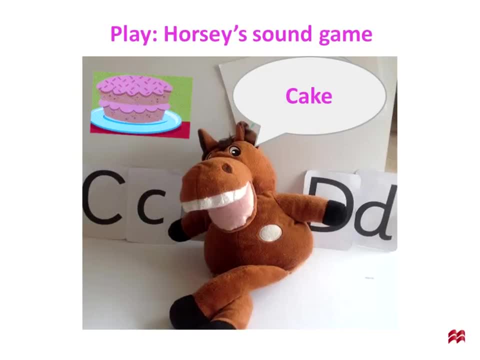 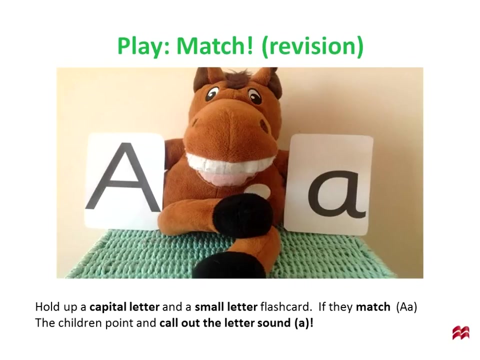 on the other side of the board and get Horsey to show a flashcard and say a k or a d word Cake. Get the children to point to the cake and say the start sound k Cake And I'm eating cake. Thank you very much for that activity, Horsey. 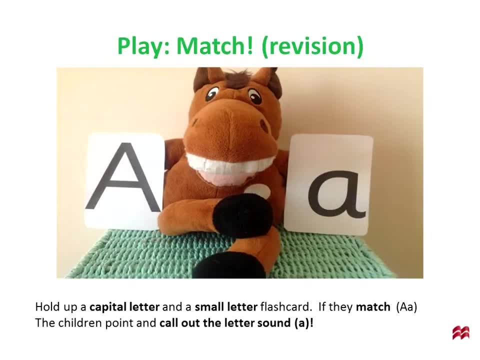 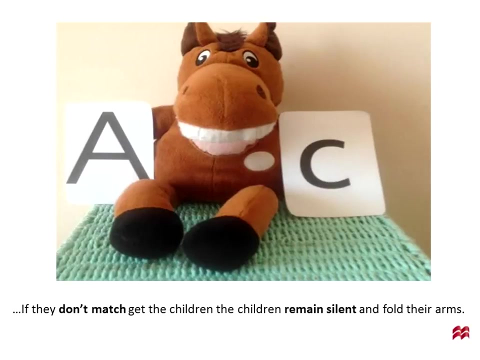 Now Horsey wants to play match. This is a good revision activity, So hold up a capital letter And a small letter. If they match, encourage the children to say the sound: Ah. If they don't match, the children just remain silent. 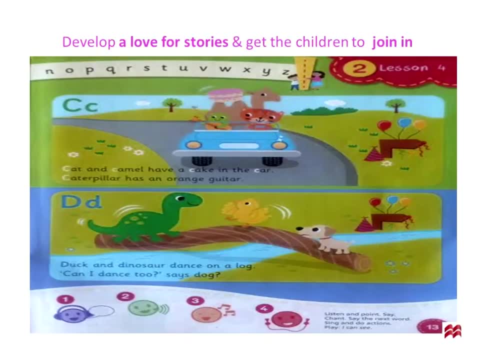 Okay, let's move on to the next, the second Fonics lesson with k. If you just take a minute to think, how did you learn to read? Just take a minute to think. Probably you read with an adult. An adult modelled reading showed you how to point from. 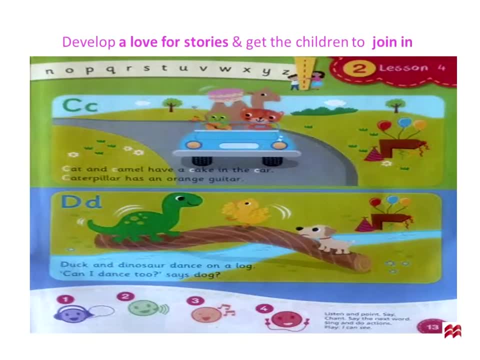 left to right. You acted as a reader and joined in through memory. Okay, this is more or less what we're doing here. This is a cumulative rhyming story and it's about animals going to a big party. Okay, this is the second phonics lesson. 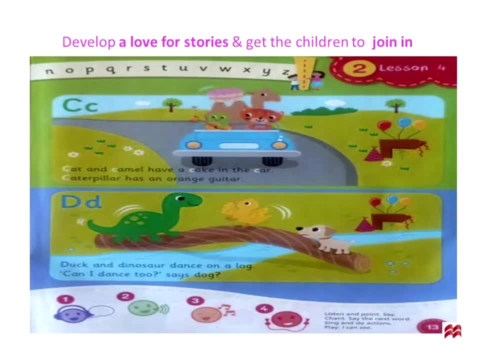 Can you tell me? look at the k picture. what can you see beginning with k: Cake, camel, point, caterpillar, cat, car. Good, Where do you think the animals are going To the party Now? how do you know that? 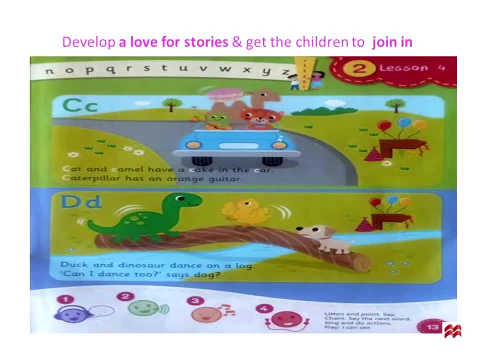 There's a party Ow Good Again. we're going to get the children to listen to the little rhymes and you point showing how the text works, pointing from left to right, And then we get the children to join in. 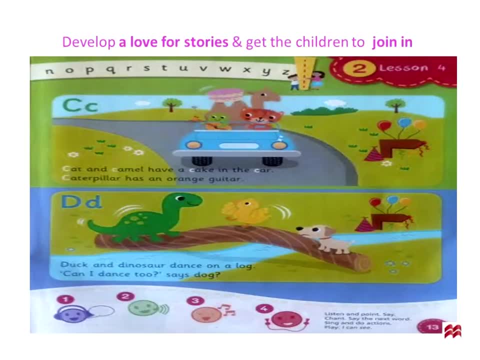 and point in their books. Let's try. Cat and camel have a cake in the car. Caterpillar has an orange guitar. How many words can you see that begin with k? One, One, two, three, four, five. Okay, can you see the k words? 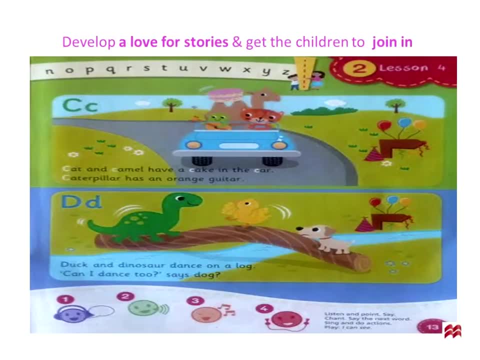 K cat and k camel have a k cake in the k car. K caterpillar has an orange guitar. Well done. Now we can get the children to stand up and do actions. Okay, Cat, perhaps Pull out imaginary whiskers. 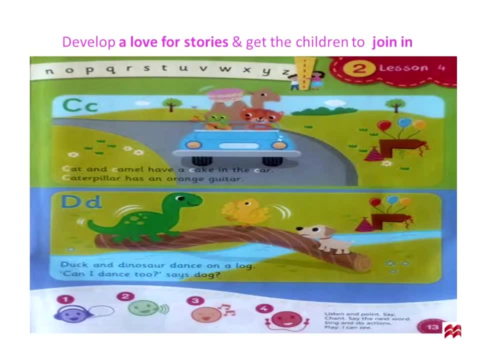 Cat and camel have a cake in the car. Mine driving a car Caterpillar with your finger has an orange guitar. Fantastic, Quick question: How many words can you see that begin with k? One, Two, Three, Four? 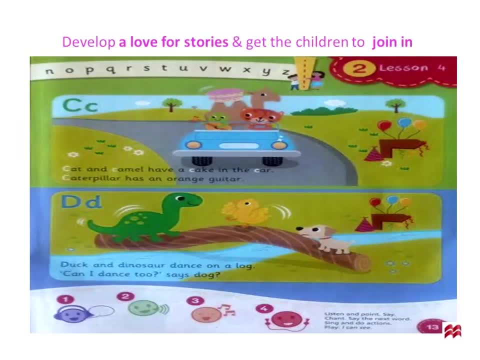 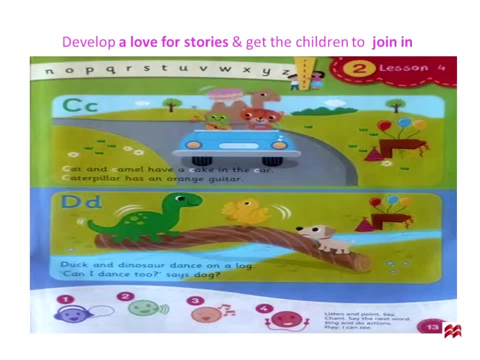 One, Two, One, Two, Two, One, Two, One, Two, One, Two. Which word rhymes with guitar Car? Very good. Who has got an orange guitar caterpillar? Very good, Now we can play. I can see. 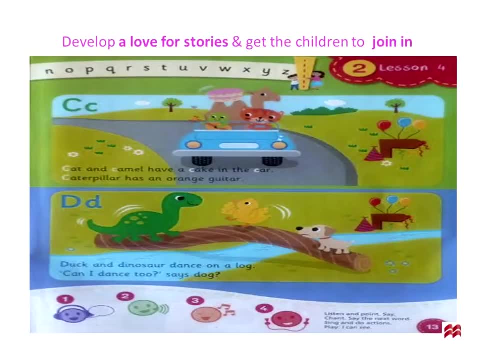 This is a little bit like I spy. So we get horsey or your puppets point to K It's a camel, Get the children to point to camel, And then we can ask a volunteer to do this and say I can see, K It's a car. So we are developing a love for reading Children. 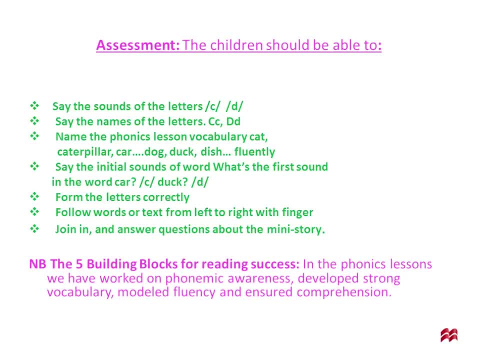 are acting as readers and recognising initial sounds. So assessment is very important And, for example, after this lesson of K and D, the children should be able to say the sounds of the letters. K, D Say the letter names, C, D, Name the phonics Lesson vocabulary. 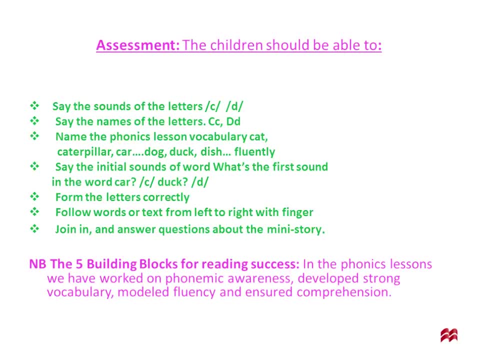 cat, caterpillar, dog, duck. Say the initial sounds of a word. What's the first sound in car K? They should be able to form the letters correctly: Capital and small letter. They should follow words and text from left to right with their 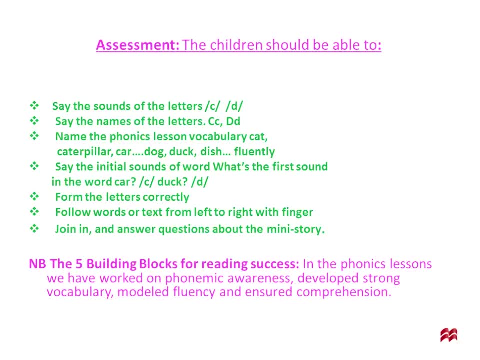 finger And they should be able to join in and answer questions about the mini-story. Now you'll notice that we have covered the five building blocks for reading success. So in the phonics lessons we have worked on phonemic awareness, developed strong vocabulary. 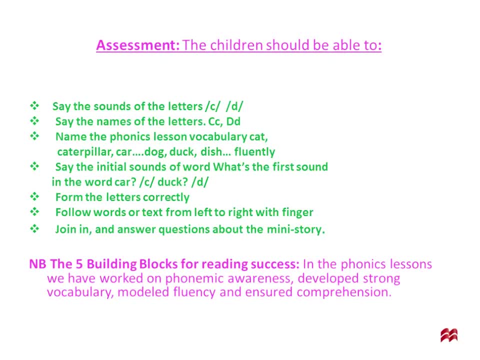 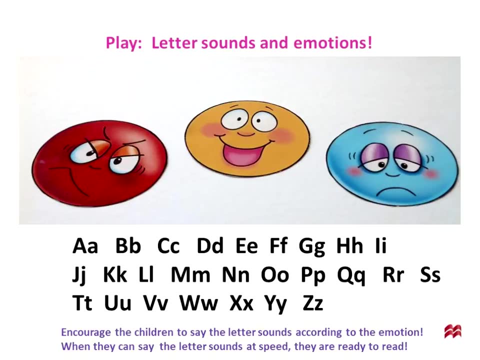 modelled fluency and ensured comprehension. Now, when the children know the 26 letter sounds of the alphabet, they can go on to learning stars too. But first of all let's play letter sounds and emotions. We can say the letter sounds according to emotion And we've got to say the sounds at pace quickly. 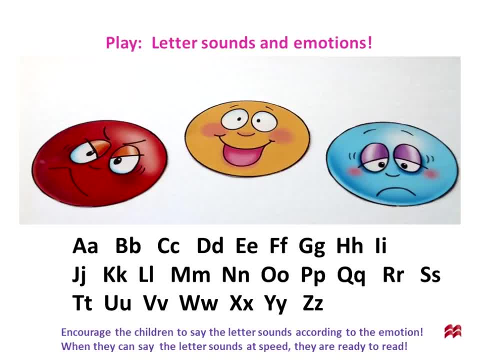 Okay, Let's all be happy, Ready Smile. Now let's see the 26 letter sounds in alphabetical order. quickly, Let's go Good, And then we can also practice out of order. And then we're ready to move on to Learning Stars 2.. 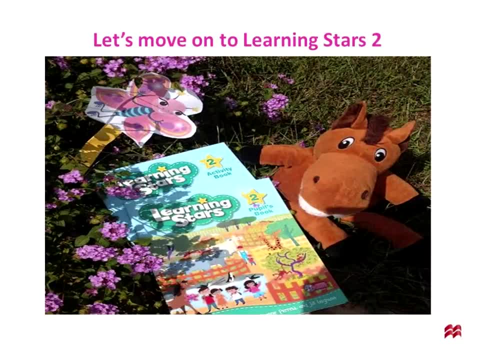 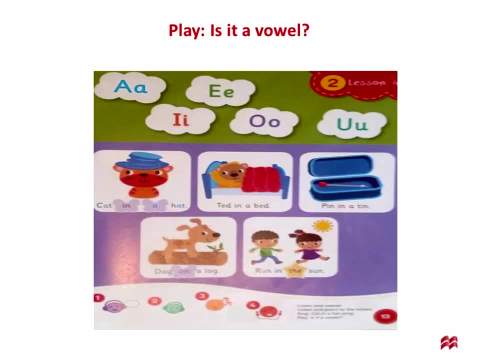 Now, here we have Bella and Horsey admiring themselves on the cover Right. Let's see. Okay, First of all, we revise the vowel sounds. There's a vowel in every word, So the children must know the sounds of these words. 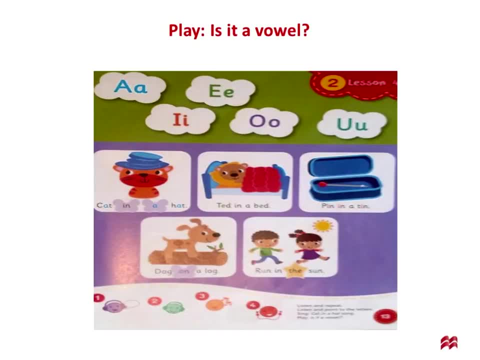 So we can make flashcards of different colours for a, e, i, o, a and stick them on the walls of our class. Then we can show letter flashcards in random order, For example d, g, e When the children hear a vowel. 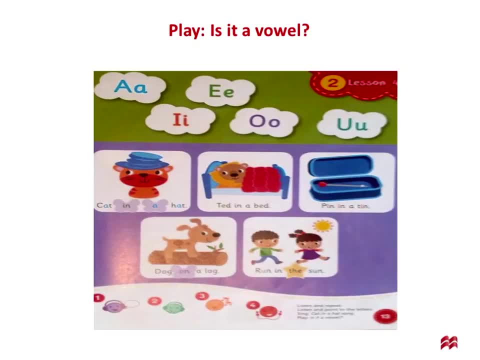 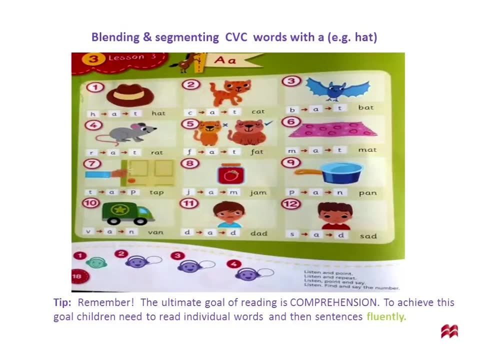 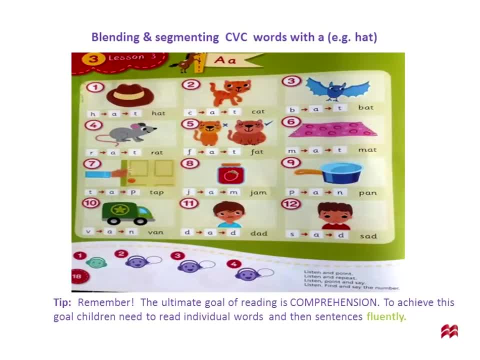 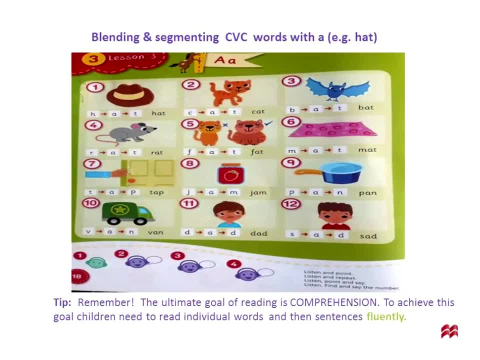 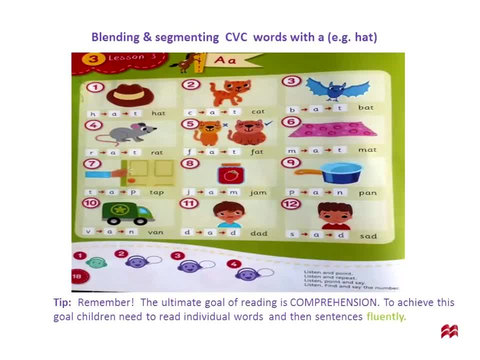 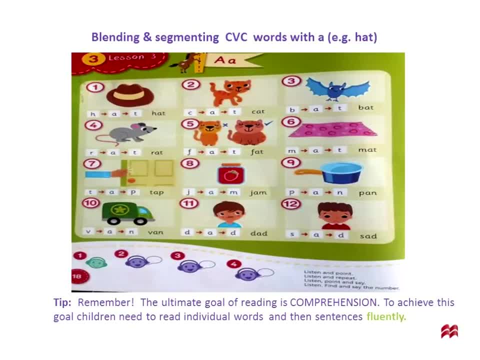 Then we can check comprehension. If you want, you can stick flashcards on the board and write the words underneath. We're going to play. find and see the number. Okay, B, J, A, M, jam. See the number. 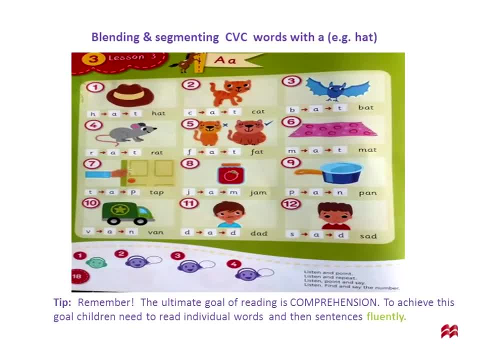 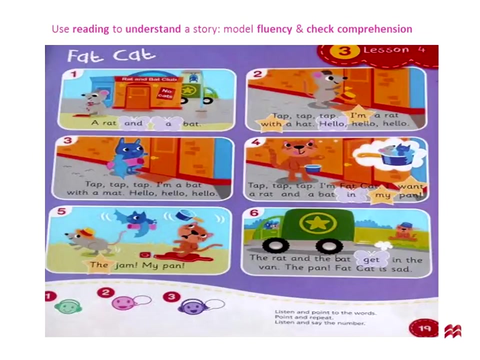 Eight F A, T, fat, Five, K A, T, cat Two: Okay, Learning Stars also has a mathematics book, so we know that they're counting well to 12.. Okay, Let's continue Now, when the children can blend consonant-vowel-consonant words with ease and fluently. 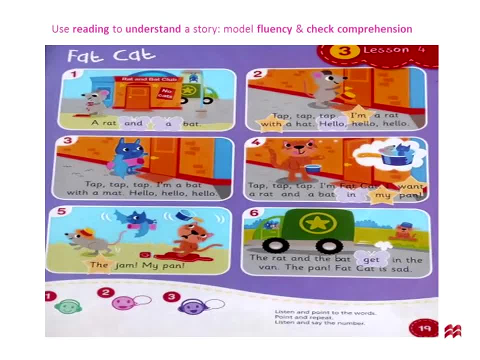 we can teach them some common high-frequency words and some irregular words so that they can use reading to understand. Now, as these high-frequency words cannot be illustrated, children don't usually pay much attention to them. So what we've done is we've outlined common high-frequency words. regular words with bella. 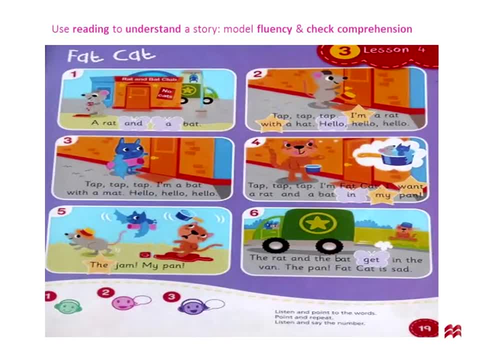 They're bella words. They can be sounded out: And, and, and. the irregular tricky words are the star words. They are star words because they star so much in the language And if the children know these words, they'll be able to read fluently. 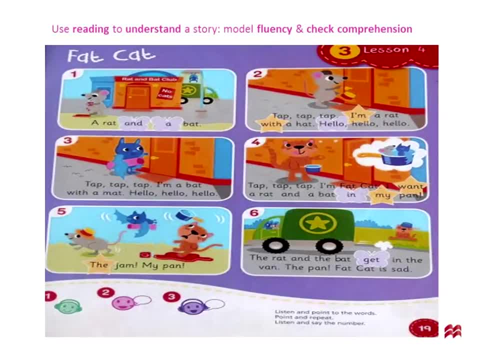 And we must practice these words a lot. So you'll see, in picture two I'm and with are marked with stars. Okay, Let's begin the story. Get the children to blend the title F-a-t-e- say the sounds, and the word fat, c-a-t-e. cat, fat cat. 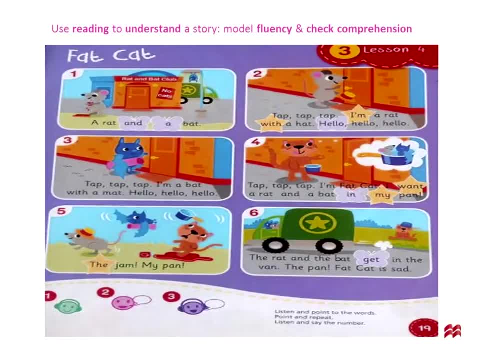 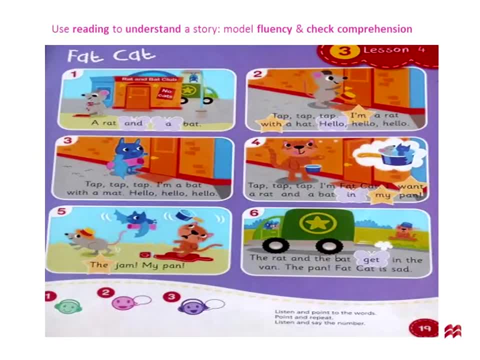 A cat, A cat, A van Jam Who has spilled the jam Rat. Very good. Is this a football club? No, It's a rat and bat club. Look, it says no cats. Why? Why does it say no cats? 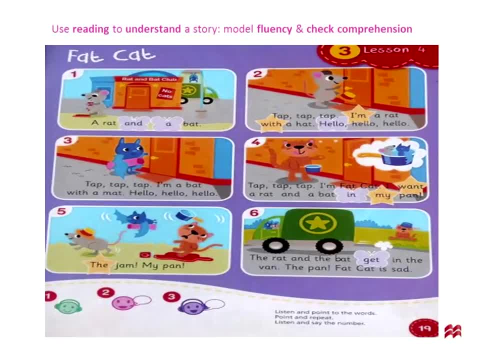 Yes, because cats, Cats like to eat rats and bats. Let's have the story And we show how to point to the words from left to right, And then the children would join in the story. Okay, A rat and a bat. 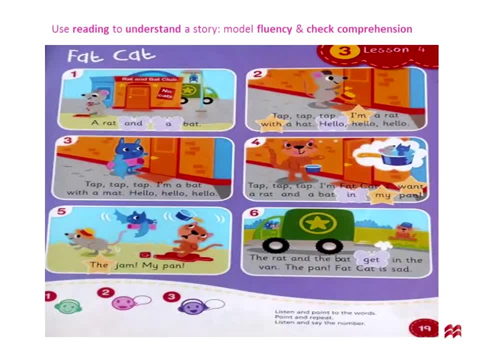 Squeak, squeak, squeak, Tap, tap, tap. I'm a rat with a hat. Hello, hello, hello. Tap, tap, tap. I'm a bat with a mat: Hello, hello, hello Meow. 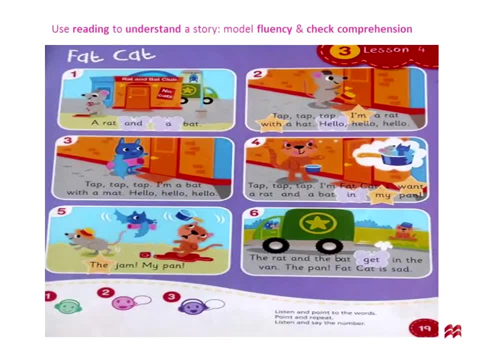 Meow, Tap, tap, tap. I'm fat cat, I want a rat and a bat in my pants. I'm hearing a meow, Squeak, squeak, squeak. Ooh the jam Meow. 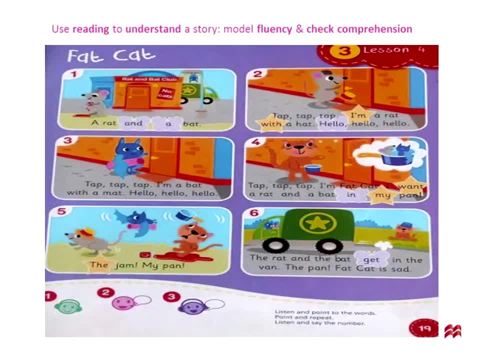 My pants. The rat and the bat get in the van Vroom, vroom, vroom The pants. Fat cat is sad. Oh now, why is that cat Sad? Does he have a rat and bat in the pan? 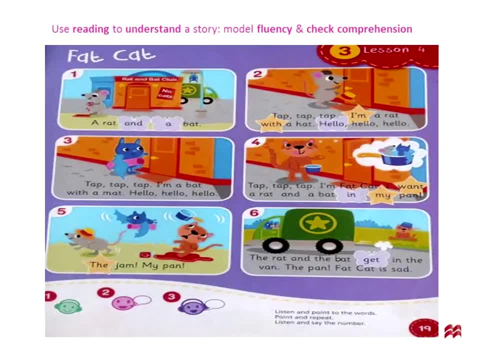 No, What's on his head? The pan. Very good, Now we're going to get the children to listen and say the number to check for comprehension. Listen A rat and a bat. Say the number: A rat and a bat. 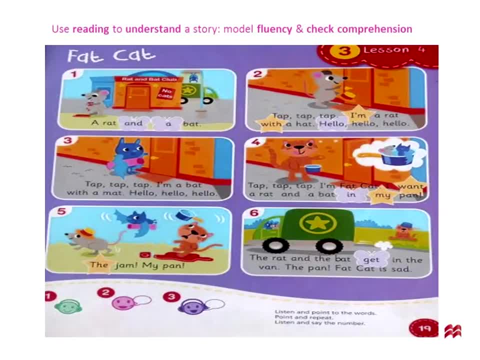 Say the number, My pants Say the number. Okay, They say rat and bat, One The jam. My pants Say the number Five. Very good, Can you look at picture four? How many star words are there? Two: 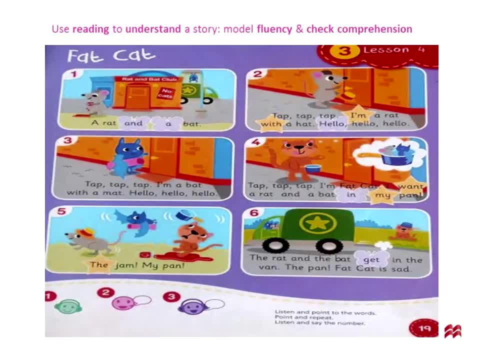 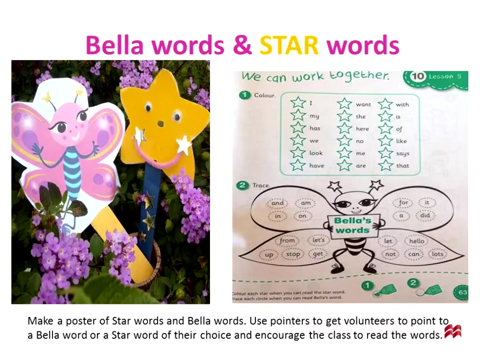 Can you read the star words? One My Fantastic. Look at picture six. Can you see a bill-O-Word word? Let's sound it out. Get Well done. We can read better words and star words. You may wish to make a poster of irregular words, common irregular words and common regular. 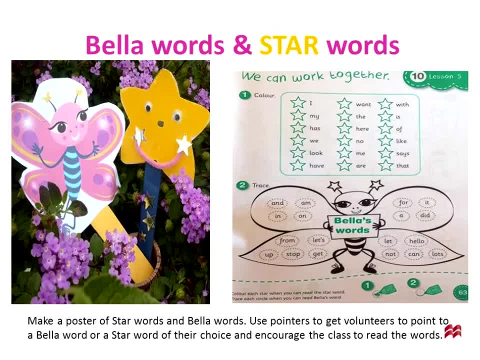 words. So we have here two pointers: A pointer of Bella and a pointer for star words. Get the children to choose a pointer, For example the Bella pointer. Get one child to point to Bella words and the rest of the children can read the words And am in on Then. 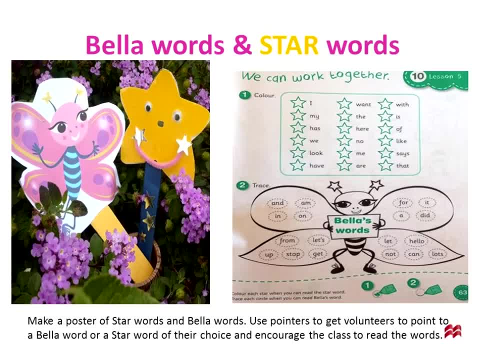 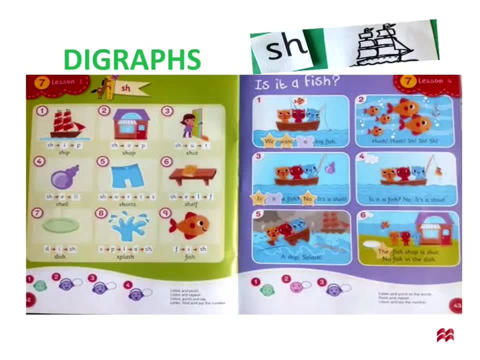 get the child to take the star pointer and point to words like I want And with Okay. Now a word on digraphs. Digraphs are two letters that make one sound. For example, shh Ship begins with shh, S begins with shh. 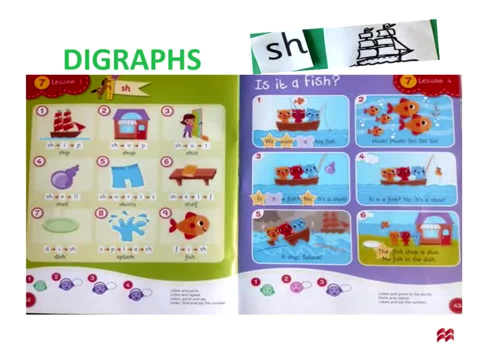 H says shh, Two letters, one sound. We can play flashcard games like sequences with the children, with the flashcards first. For example, flash Ship, ship, ship, Sh, sh, sh, sh, ship, Sh, ship. Okay, Now here we can see that we're going to practice shh. if you look at, 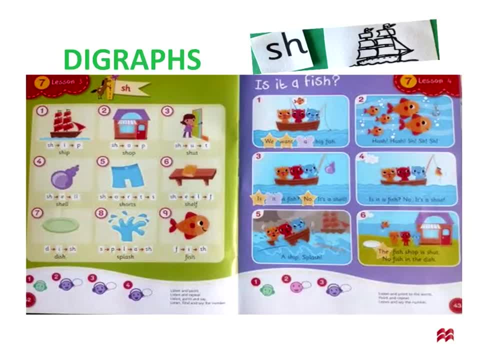 the banner. We read the words The same way. We just blend Sh e, p, Say the sounds, then say the word Ship Sh o p, Shop Sh a t Shut. Children need practice, And what we're doing with our chants is we're modeling how to read. 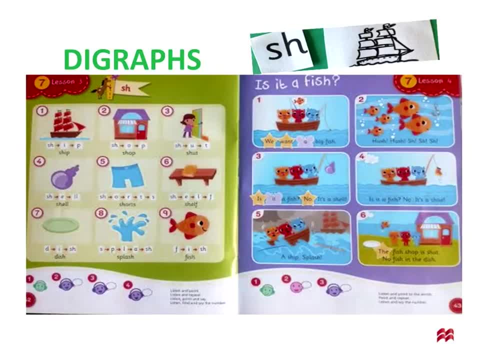 words. We can say the word without gaps: Sh e p Ship, Sh o p Shop, Sh a t Shut. Then we can get the children to spell the words So they hear the word ship and tap out the. 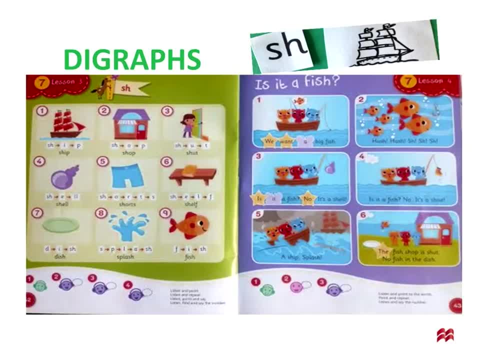 sounds: Sh e p Ship Shop. Sh o p Shop. Sh e p Shop. Sh o p Shop. Sh e p Shop Shut, Sh a t Shut. 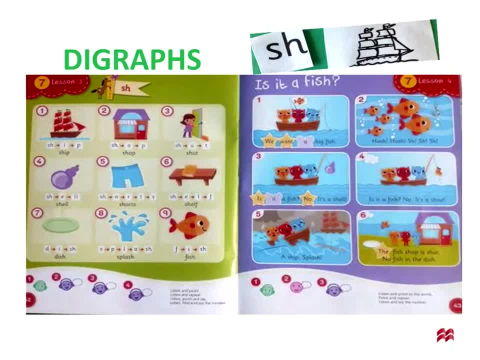 Shut And then again we can play. say the number, making sure they're understanding: Sh e p Sh fish Say the number Nine. Sh e p shell Say the number Four. a sh This. 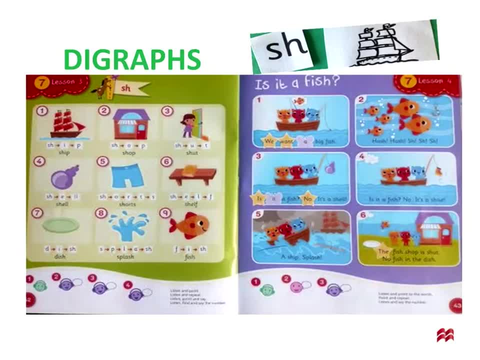 says a number Seven. Okay, Now we're going to go on and have a decodable story with the sh sound. When I read the story, you can clap when you hear the sound Sh. This is a nice activity that you can do with many. 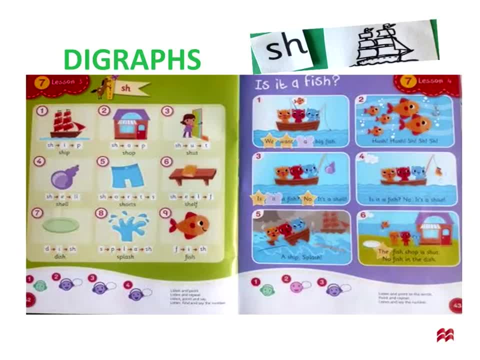 stories. Okay, Again, read the story. Blend, blend the sounds. Is it a fish? Is it a fish? We want a big fish. Meow, Push, Push, Shh, shh, shh. Is it a fish? Meow. 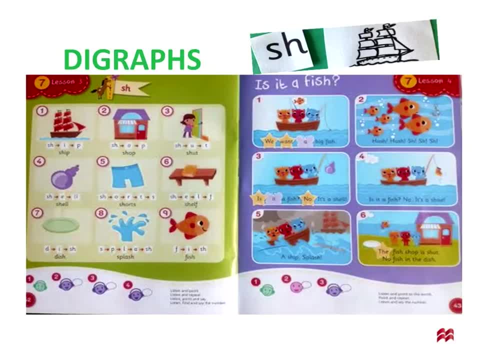 No, it's a shell. Is it a fish Meow? No, it's a shoe. Oh, a ship Splash Meow. The fish shop is shut And there's no fish in the dish Meow. Are the cats happy or sad? 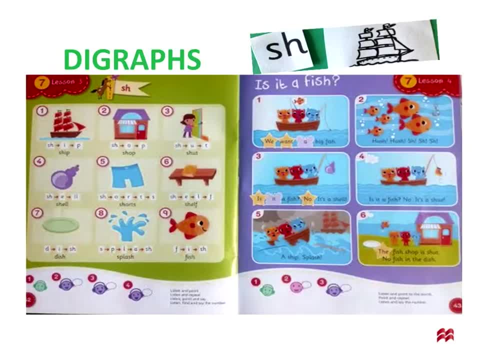 Yes, they're sad Why The fish shop is shut And there's no fish in the dish. Can you tell me a word that rhymes with fish Dish? Well done By modeling how to read. the children will soon be reading the story. 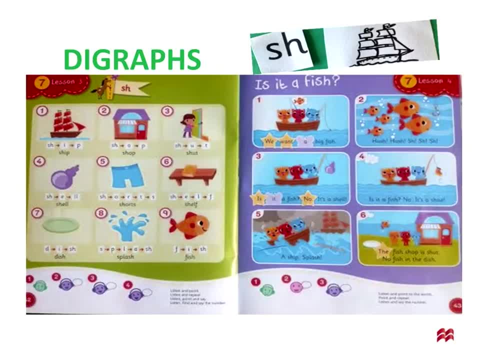 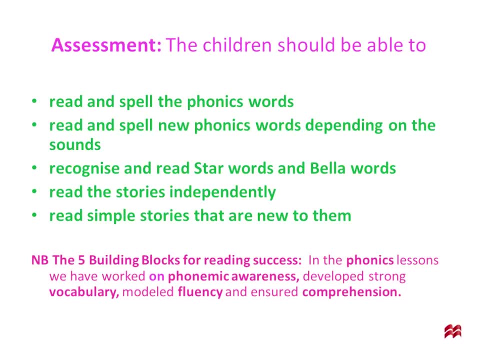 Well done By modeling how to read. the children will soon be reading the story. I'm sure they'll be reading fluently on their own. I'm sure they'll be reading the story Now. assessment: At the end of Learning Stars, Level 2,. the children should be able to read and spell phonics words. 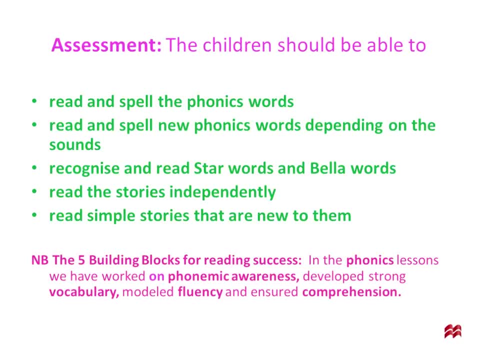 Read and spell new phonics words depending on the sounds. Recognize and read star words, irregular words and bella words. high-frequency words. Read and spell new phonics words depending on the sounds. Recognize and read star words, irregular words and bella words. high-frequency words. 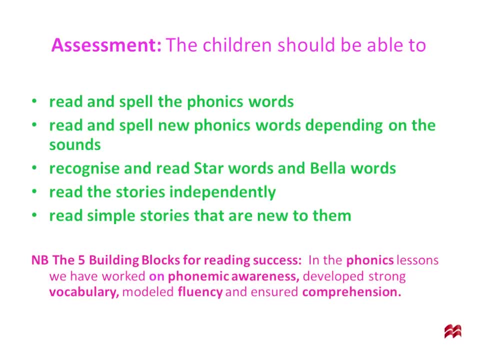 common words. they should be able to read the stories independently and they should be able to read simple stories that are new to them. So if we think back to the research for successful learning, we have covered the five building blocks for reading success and in our phonics lessons we've worked on phonemic. 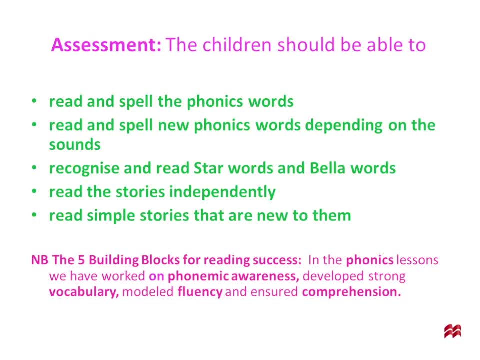 awareness, developed strong vocabulary, modelled fluency and ensured comprehension. Wherever you're teaching in your phonics lesson, it's always good to get the children to look at your mouth. The puppet is great for games, but to show the children how to say the sounds, they should look at your mouth. 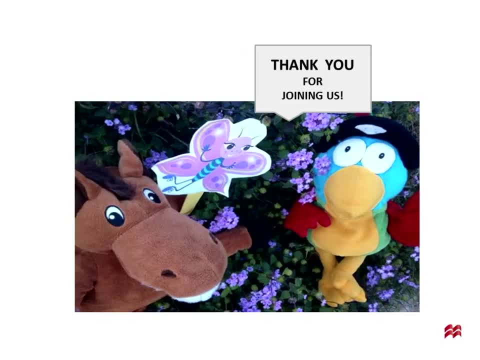 Okay, so thank you for joining us. Thank you, And I hope this has been useful. We have taken three-year-olds to five-year-olds to the stage that they can read, spell and write and they're ready to go on to the big school. 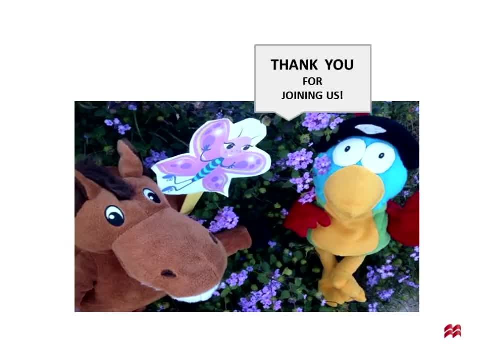 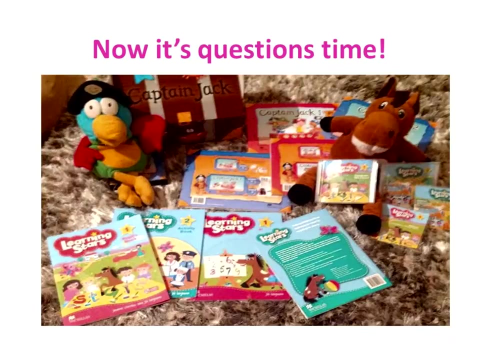 Okay, thank you very much from me, Jill, Leighton and Horsey. Captain Jack, Thank you for joining us. Okay, so now it's questions time. That's right everybody. Okay, Henry, Who enjoyed the session? I did, Horsey did. You're very excited now because it's time for questions. Yeah, Horsey likes questions. 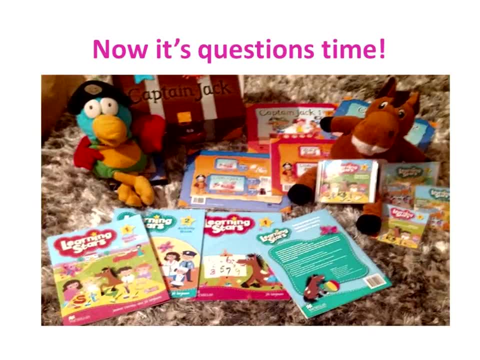 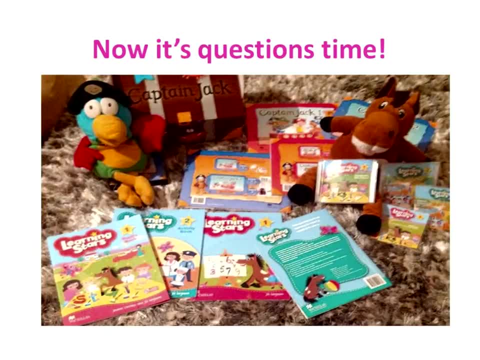 Oh, it's going mad, Okay, Oh right, Jill, I'm just reading some of the things that are coming in: Certificates: everyone. they'll get sent to you later today. Rodrigo is wondering if you could apply the same concepts to teaching children another language. 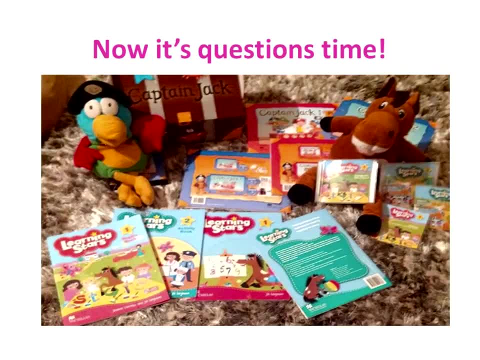 You don't have to be a teacher to do that, but I think that's what all of them are doing, Or using the material, for that matter. I don't know if that's a right question. I imagine What's the language? Rodrigo, write to us in the chat box if you want to know. 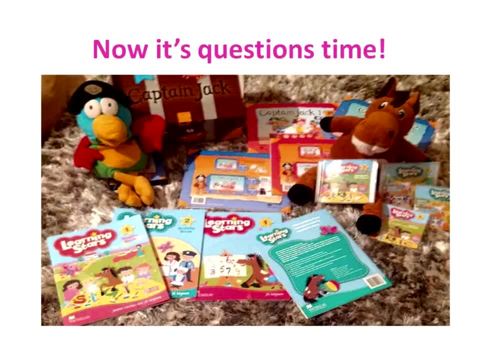 Okay, Okay, Rodrigo's disappeared. Oh, hmm, Don't worry about it. get Rodrigo to come back later. Mark, he wants to know what are the star words. again, I think the star words are common irregular words, for example the I with the children. 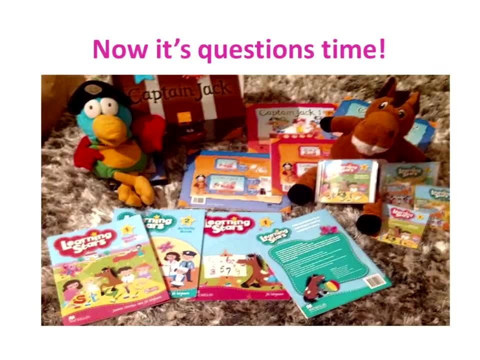 need to learn star words to be able to read fluently. so the star words are the tricky words, common tricky words, irregular words, and can you just recap? and they star in the language. so much the star words are common, irregular. what about the bella words as well? 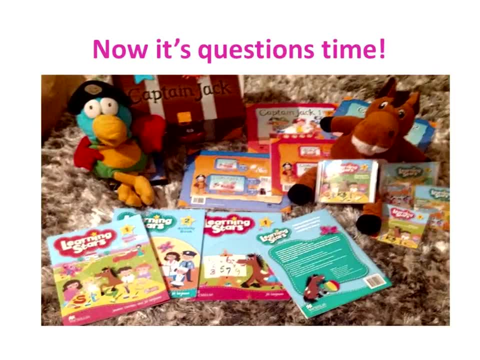 the star words have to be memorised. ok, they cannot be sounded out. the bella words are common words that can be sounded out, for example: and so bella words. the children can see the sounds and sound them out. excellent, I think that clears things up. yeah, Mohammed wants to. 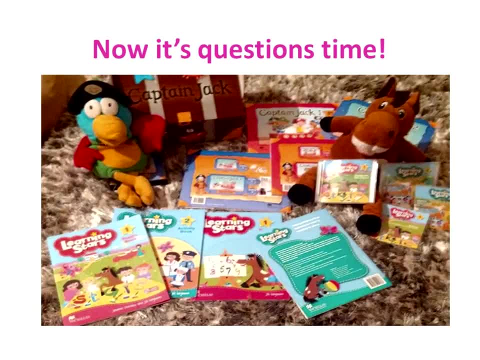 know how long you should spend on using these methods in class. how many lessons are usually needed to get young learners up to speed? well, in learning stars there are ten units and in each unit there are two lessons. so over the two years of learning stars, perhaps you have. 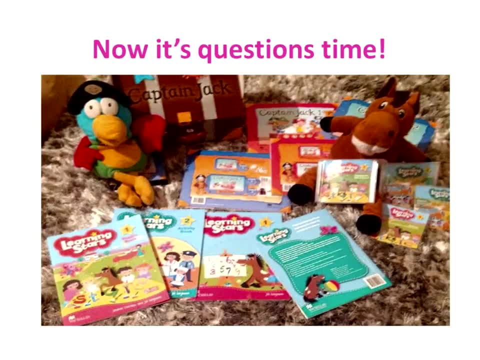 it's very flexible, from four hours a week to eight hours a week, with the community to decide as well, plus the phonics and what we we could get the children reading and spelling in two years from three to five year olds. great thanks for that one, Jill. 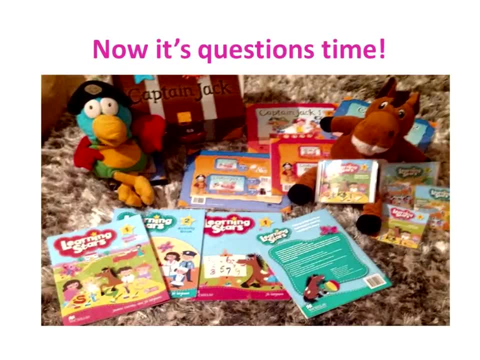 we've got time for one more question, I think. thank you, so let me see. write your questions in now, guys. if you need an answer, okay, I'll just wait a few moments to see what comes in. Tamir has a question. go on, Tamir, write your. 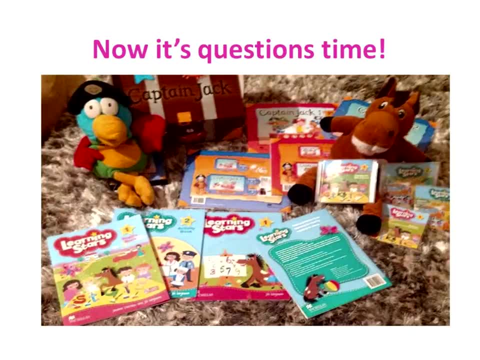 question in the box if you want to get it answered by Jill now he's typing. okay, Tamir, sorry, Jill, just waiting for everyone to finish typing. if anyone didn't get their question answered, you can email us and contact us as well. I'm putting the address. 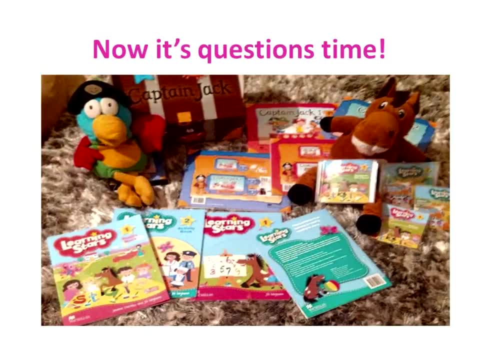 in the chat box, and a good thing to check out would be the website, the learning stars website. yep, that's it: learning stars website, which my colleagues have been sharing with you in the chat box. Julie and Carol have been putting all the links in there and this: 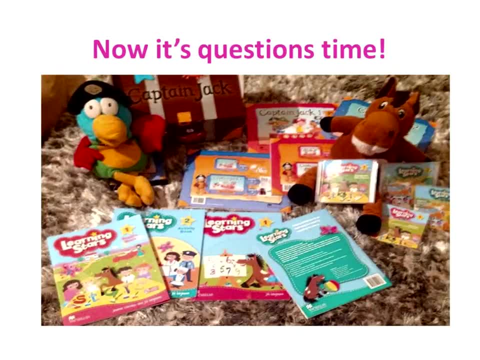 presentation is going to be available to download next week and we'll have the links to everything in there for you as well, so you can take a good look at it next week in your own time as well. let's see if there's any more questions in here. 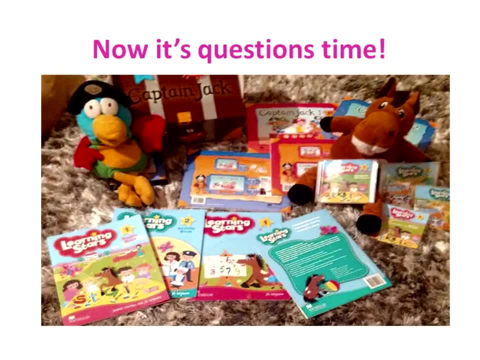 right. last question Jill Valeria wants to know: is spelling more important than pronunciation when teaching young learners? what's your opinion on that? well, I think, Valeria. I think it's all interrelated. we have to teach children phonics so that they can spell correctly, and we're